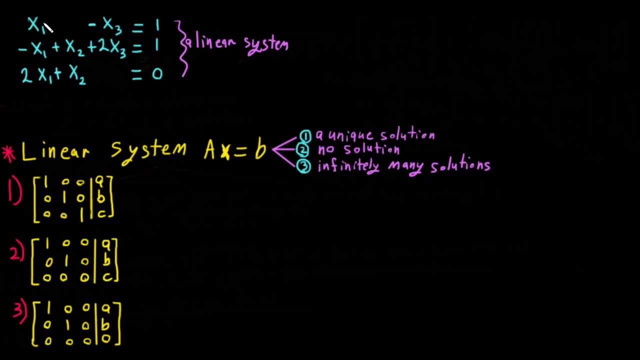 three, a linear, because we know from the previous video, here it's order one here, all of them order one here for one bar on bar one, and maybe you asked me where is these two? maybe it's not one, of course, here it should be one, it's look. 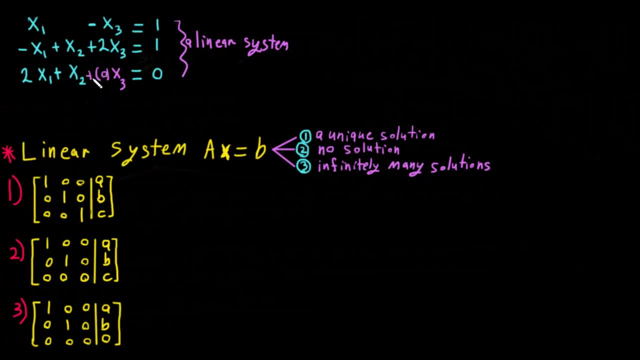 like this, but it's multiple by 0 plus or minus, so that's why it's vanished here and same of this one. that's why it's there is nothing here, because it's multiplied by 0, so it's it's vanished from here and here. so here it's a linear system, of course, if, if you want, 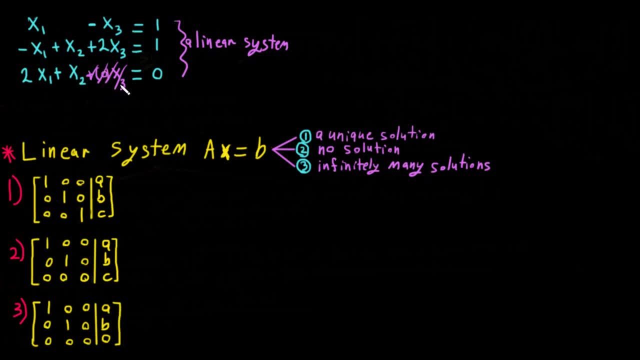 to write it in your essay or in like to describe the system. it's better to to call it something, so that's why we called it this one sometime. be it's equal to 0, so we will write ax equal 0, but this one we will tell you later. so 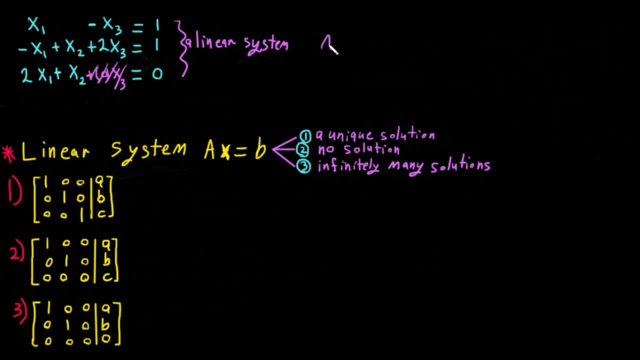 here we have what is a- I'll write it here- a equal. it should be the same size of this one. so one two, three, one two, three, one two, three. so nine element here should be here. nine element here: one zero minus one minus one. one two, two, one, zero. okay. so, of course, if I want to, 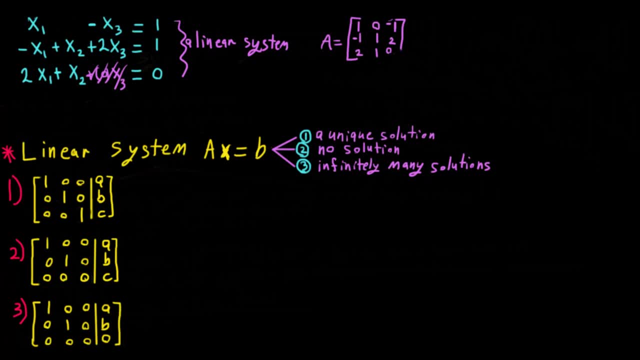 here is this one, so it will look better. so here, better now, okay, so here the zero. so these, we have three rows, three columns. we have three column here, three row, but we don't account this one because we only, we won't write this one and this a, and you know, here a, it's only. 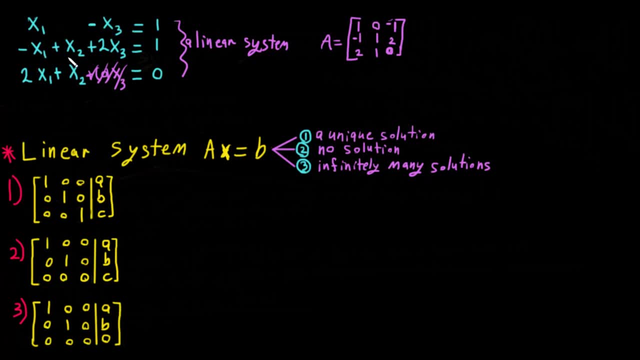 coefficient here 1, 0 minus 1 minus 1, 1 it's only coefficient. so a, what's a? a is coefficient. they called it coefficient coefficients matrix. okay, what is X- X? we have various. what is X- X, we have various. what is X- X? we have various variable here: one, two, three, we have. 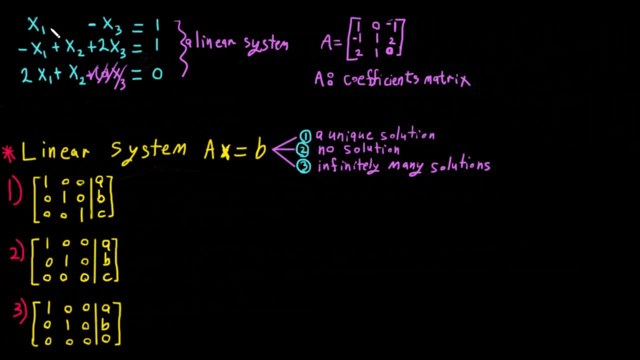 variable here: one, two, three. we have variable here: one, two, three. we have only X 1, X, 2, X 3. if you don't want to only X 1, X 2, X 3, if you don't want to only X 1, X, 2, X 3, if you don't want to account this one, account only this one. so 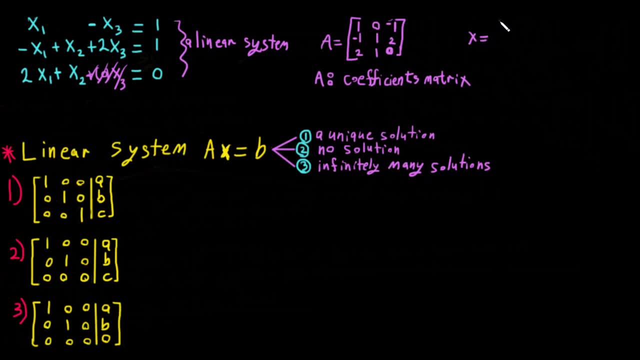 account this one account, only this one. so account this one account, only this one. so here equal X 1 X 2 X 3, and sometime here equal X 1 X, 2 X 3, and sometime here equal X 1 X, 2, X 3 and sometime more. this only example here. I put here. 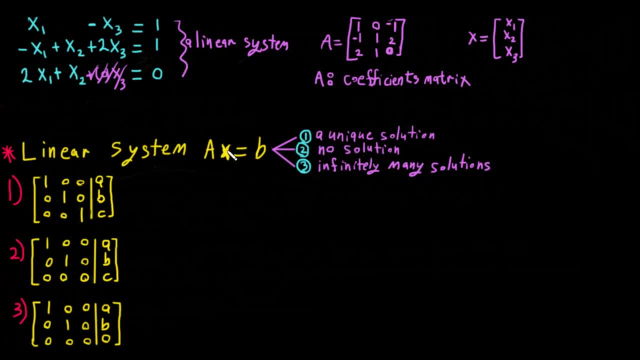 more. this only example here. I put here more this only example here. I put here, only for illustrates, what this one mean, only for illustrates, what this one mean, only for illustrates, what this one mean. so sometimes you have no, so sometimes you have no, not until x3, maybe until x2 or until x7, it doesn't matter. so here here we have x, what is x? 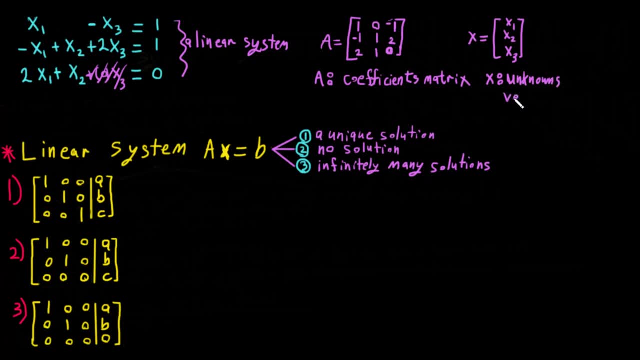 and now, or they called it variable, okay here, unknown here, k this, k, okay, what is b? b, of course the result from here, the answer of this one, so b, equal one, one zero, so b. i want to call it result or answer for the answer of the system. so here we have three things we have to know. 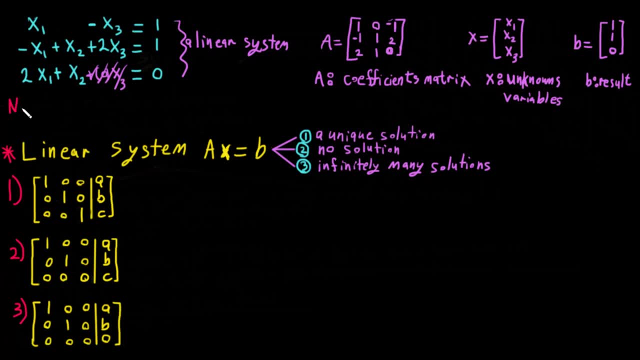 and i have here important, not not important, you can only to understand this more better. so the first one number, this i will write number: number of column here: one, two, three. number of column equal here columns equal number of a noun. now it's clear. now it's clear for everyone. I think it should be clear. and here we have four. 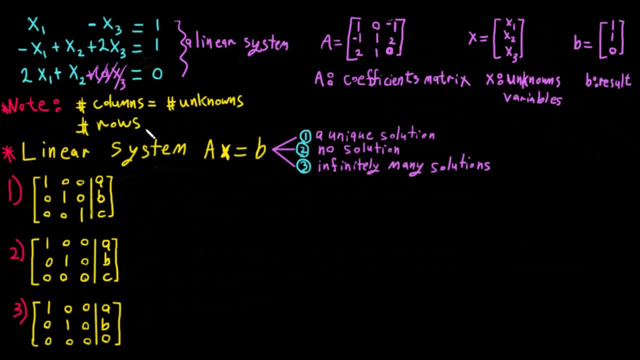 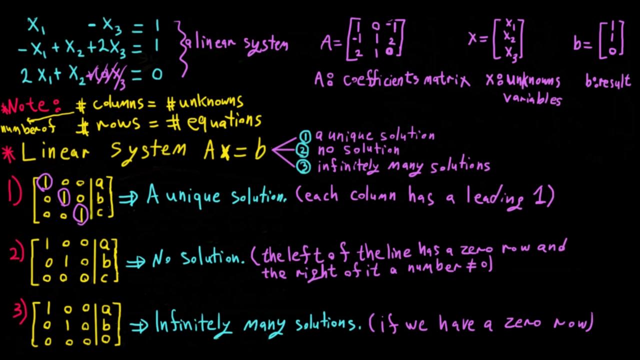 rows, numbers of rows. here, number of rows equal how many. equation we have one, two, three. number of rows equal to number of co of equation. okay, so here I mean two more straight. it's mean number, number. I like to write it in this way. so here we have three possible solution. for the first one: 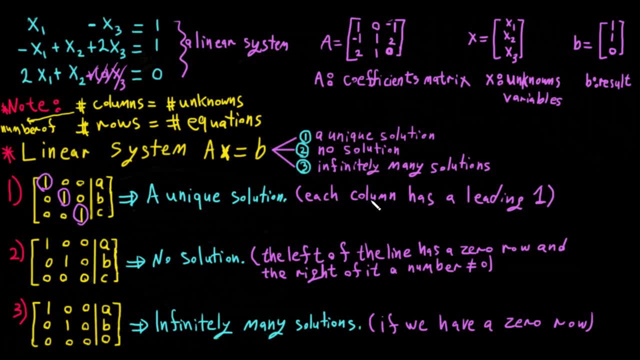 here a unique solution? if it is, each column has a leading one. so each column here, if it's- we know this, the answer of this one- a unique solution. if each column- here this one- has a leading one, and this one has a leading one and this one has a leading one. if I want to illustrate this one, why it's a unique, 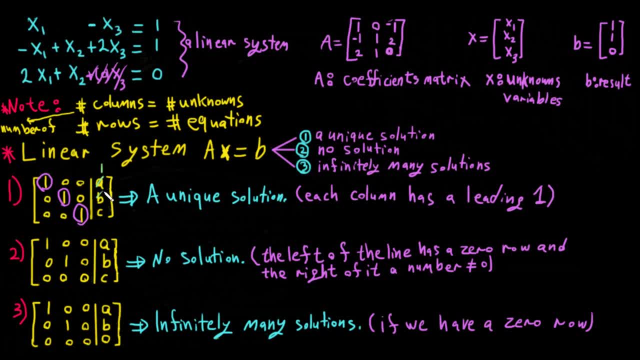 with example, let's say, this one equal to 1 and this one equal to 2 and this one equal to 2. okay, and of course we know this line represent x1, because here and here, x2 for this line and for this line, x3 for this one. here it's mean 1 multiplied by x1 equal 1. and here we 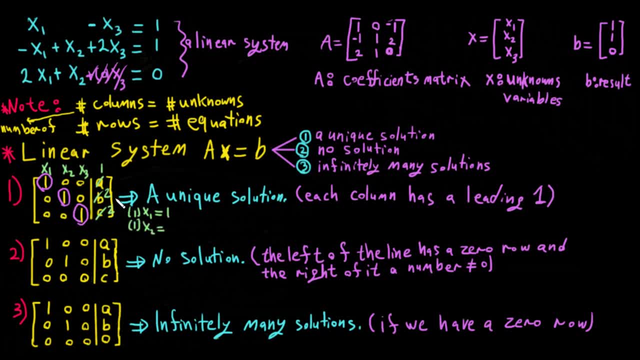 have 1 multiplied by x2 equal 2. and here we the last one. we have 1 multiplied by x3 equal 2. from here we have x1 equal 1, x2 equal 2, x3 equal 2 and, of course, from this one, we have X. when bold, I have to write it in bold: X. 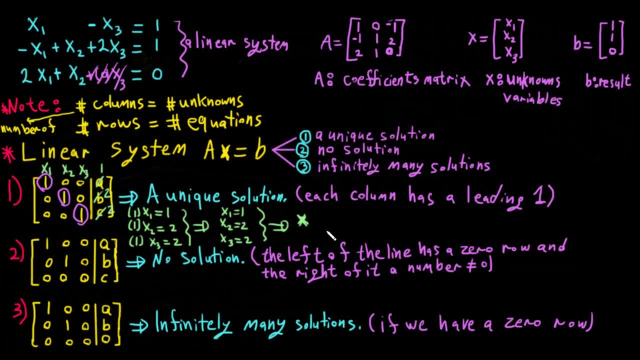 which is represent the whole thing here, as. so this one is equal to x1, x2, x3. of course, this one equal 1, 2, 2, 1 2, 2. so that's why we have only one solution, which mean is a unique solution for this one. let's say this one: if we have this shape of a, 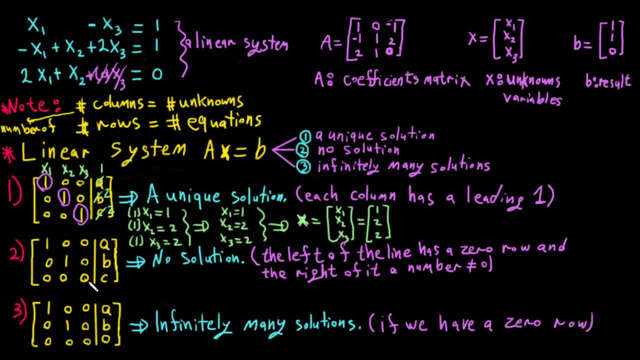 matrix. we have to say no solution because here there is a 0 row here, so the left of the line has a 0 row. the left of this line has a 0 row and the right of it a number not equal to 0. so this one it has to be not equal to 0 for. 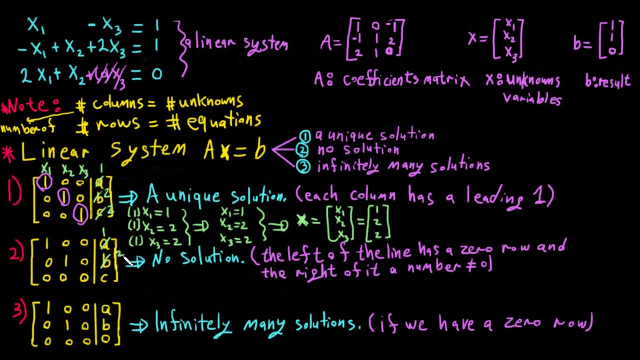 example of this: one equal 1, the same example, this equal to, and this one equal to the same thing. so here we have: 1 multiply by x1- equal 1, 1 multiply x2- equal to 2. and here we have the last one we have. 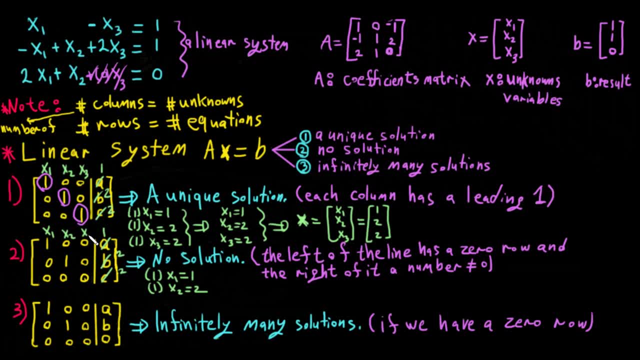 because here x1, x2, x3. for the last one, here we have 0 multiply by x3, equal to. from this one, we have 0 multiply by x3, which is 0, equal to, which is impossible, which is impossible, not 0, it's not equal to 2. that's why, from here we have, from this: 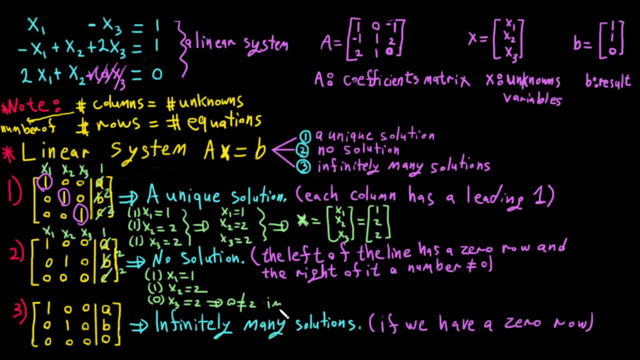 one. it's not possible, impossible here, impossible. therefore, we have no solution for the last one. we have x1, x2, x3 for the last one. we have x1, x2, x3 for the last one. here the same thing. infinity many solution if we have a 0 row on the like.